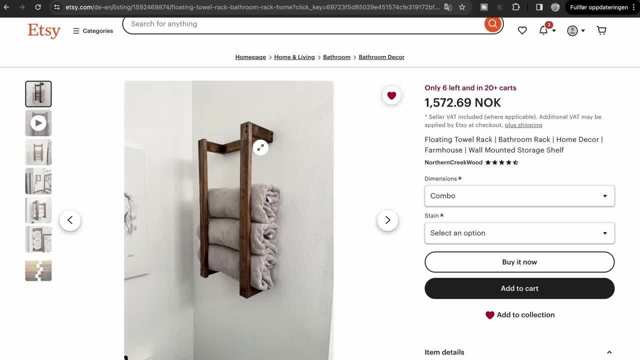 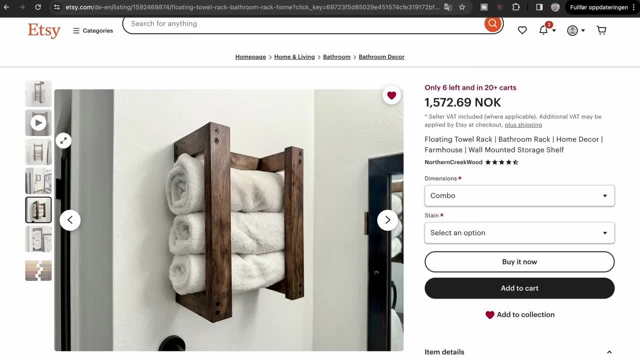 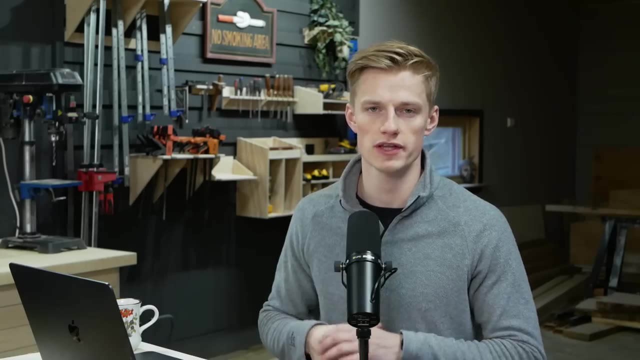 $160.. You can see, this is just eight pieces of wood, butt, joints and screws. This is a great product, pretty simple, And it looks amazing. I mean, it looks really, really good. At number two, we have what might just be the easiest woodworking project I've ever seen, And 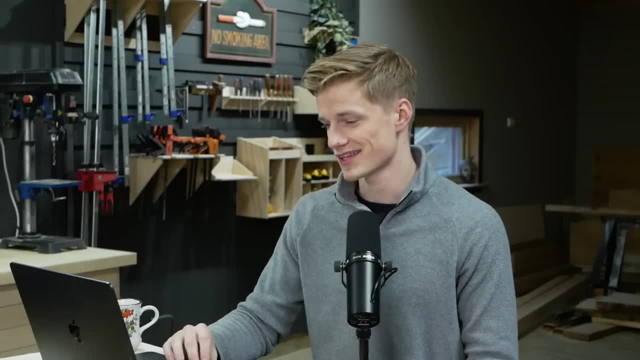 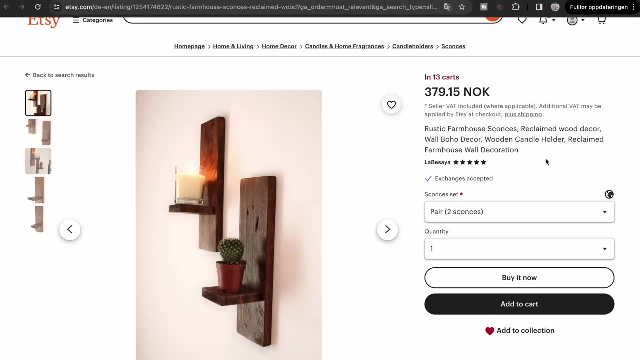 I know I've said that before, but this one is even easier. So this is a sconce candle holder. I'm not sure how to pronounce that. Is it sconce or sconce? I mean, look at this, It's one longer. 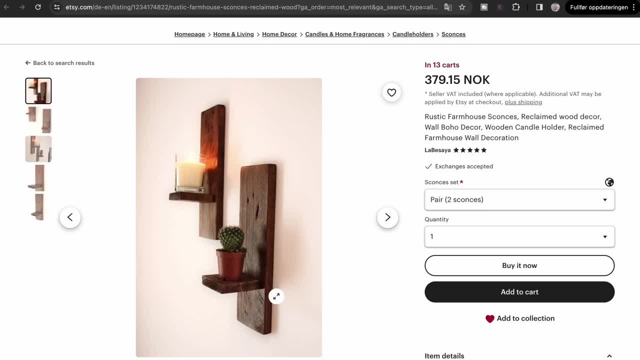 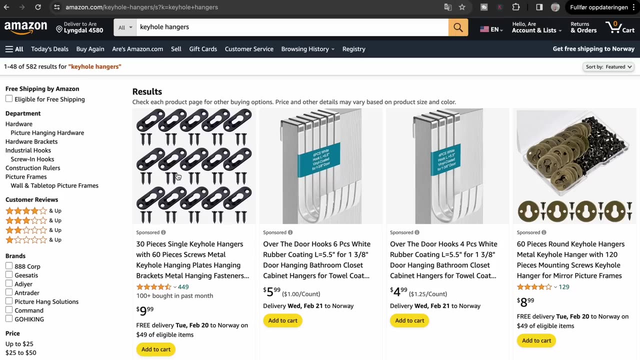 piece of wood and a shorter piece of wood, Then you probably have a couple of screws in from the back here to hold this little shelf. You can put candle or other ornaments on it. And then at the back- I would guess that they have, you know, a couple of these keyhole hangers. 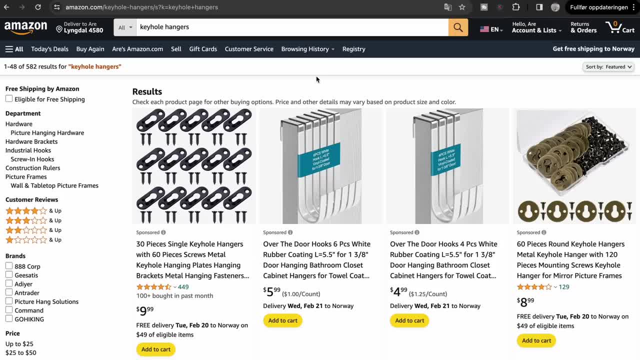 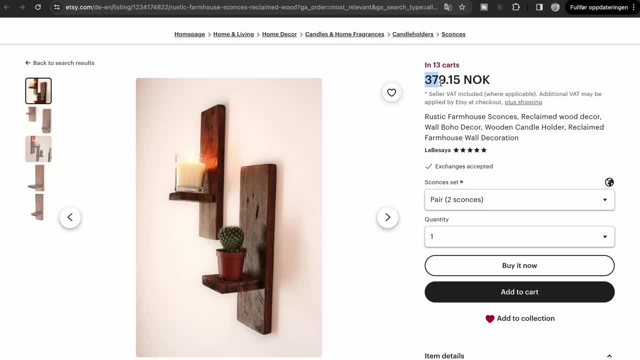 at the back So you can just hang it on the wall. I would guess it's probably 15 to 20 minutes to make a pair of these And they're selling for $38 roughly. That is for a pair If you have a single. 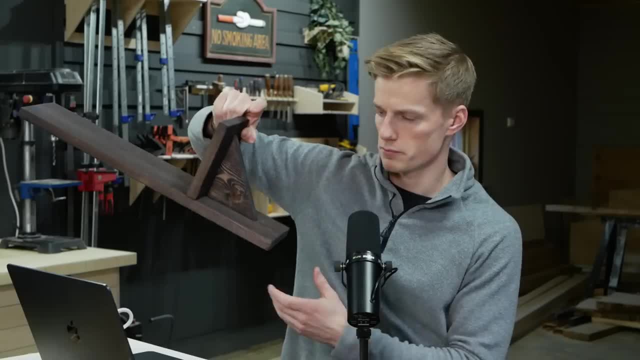 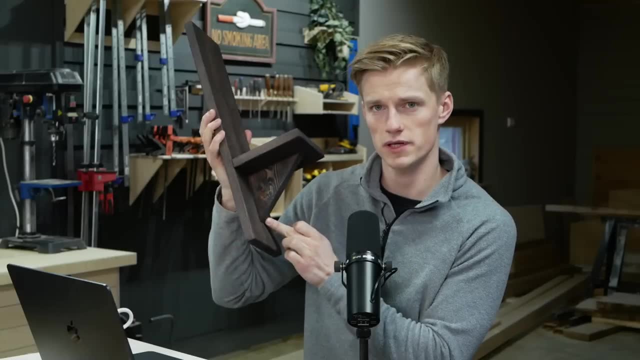 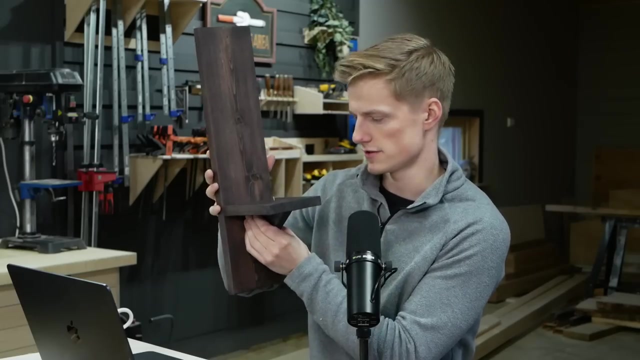 one. it's around $19.. I have made my own version of these Looks like this, So it's very similar Piece here. Hopefully you can see that. And I also added a little nail here, because what I'm going to use this for is I'm going to have a candle on top here, So I'll make some woodworking. 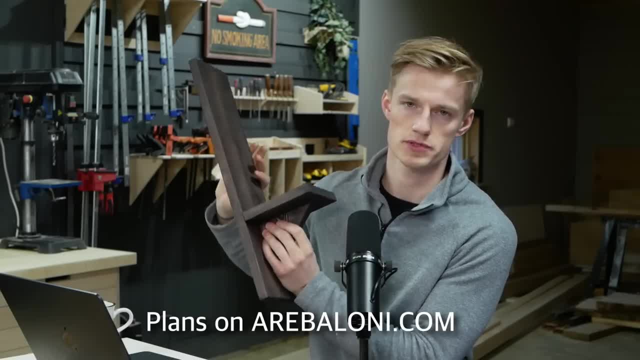 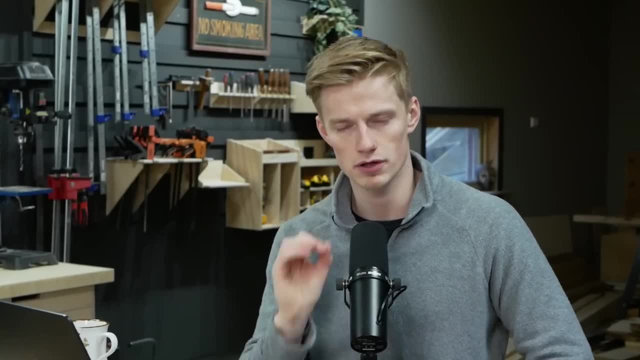 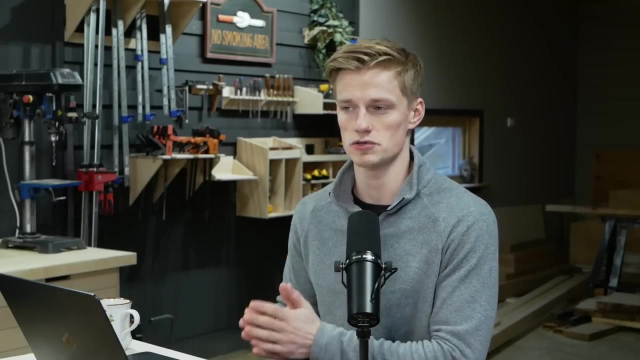 plans for these that you can download for free down in the description below. Number three is another brilliant one. This is a bestseller on Etsy and I would love to have one of these. I don't personally have a bathtub, but my parents do, And every now and then I like to use that. 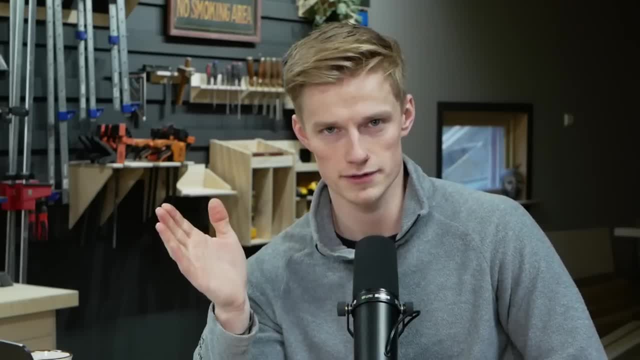 bathtub And I'm going to have one of these, And I'm going to have one of these And I'm going to. When I take a bath, I go all in. So I'm not gay. There's nothing wrong about being gay. 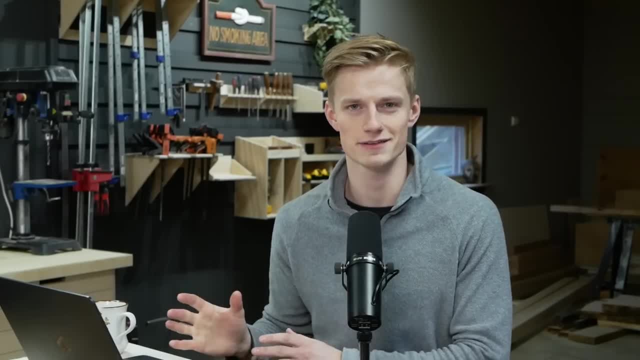 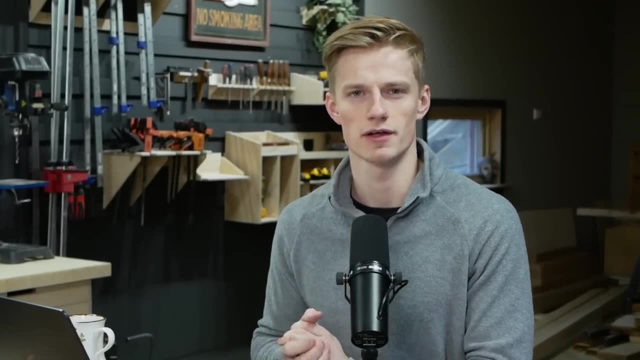 but I'm not gay, But I like to have, like scented candles. I want to have a glass of cider, maybe some snacks. I want to have a book, maybe a phone to watch Netflix or something. I want to do it properly, right, But when I do that it's always a mess because it's not really. 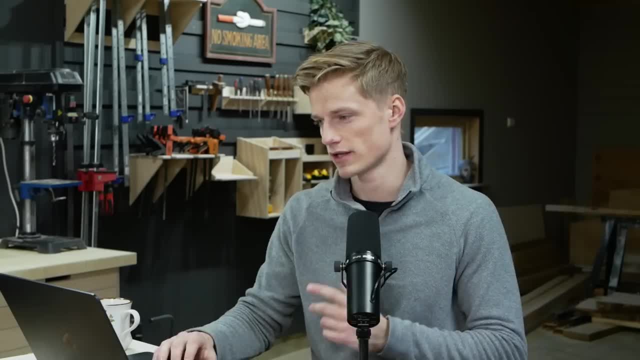 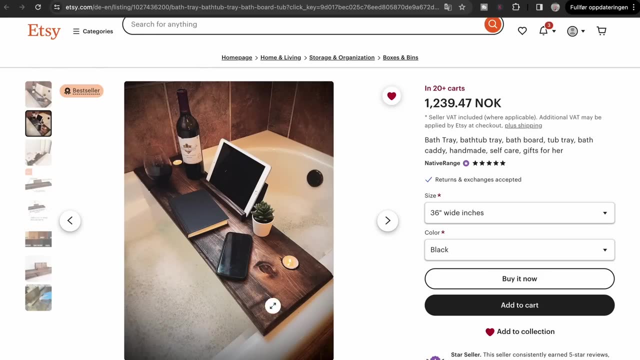 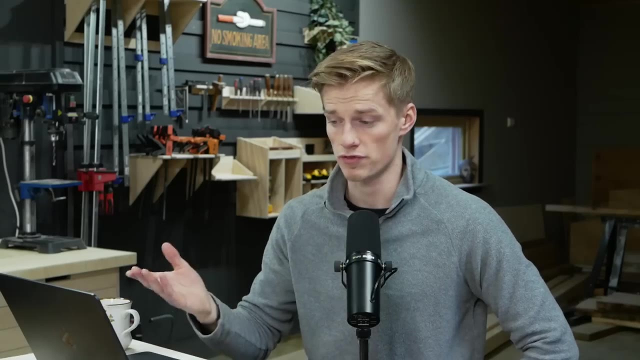 a place to have all of those things. That's where this bathtub tray comes in, And it's just a simple piece of pine. It looks like this is nine inches wide. This is again a bestseller, So this item has had a high sales volume over the past six months. So there are two candle holders, which is probably 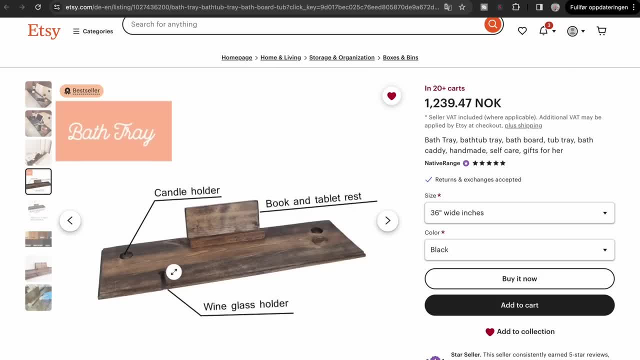 done with a forstner bit. You have the wine glass holder. It's just a hole. Then you make these cuts. You can either do it on a table saw or just using a jigsaw. Then you have this angled piece in the back and then this smaller one in the front to hold. 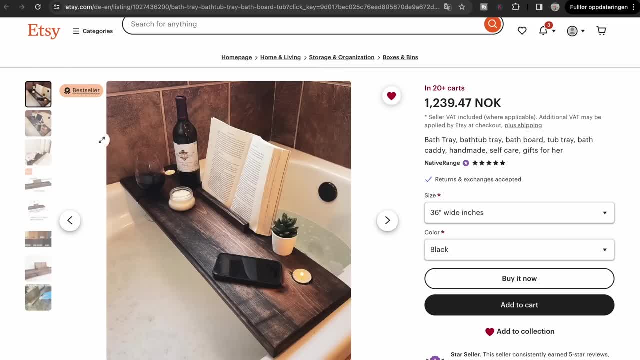 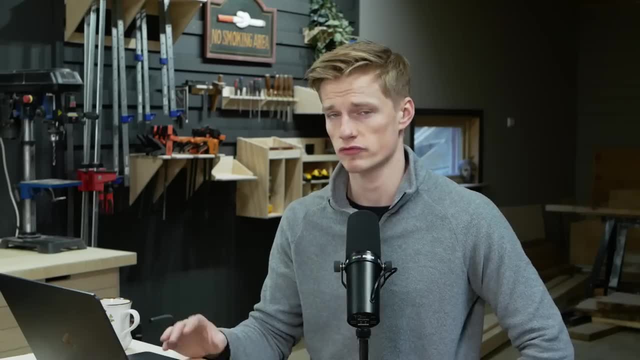 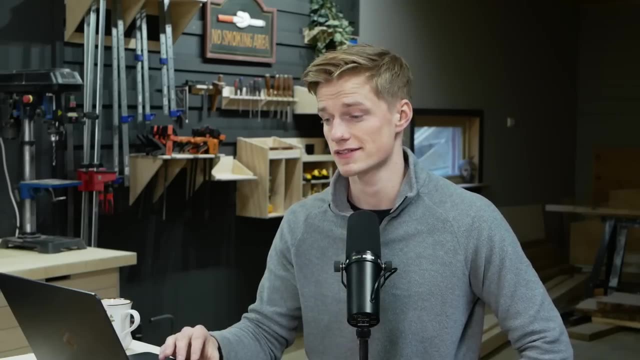 Like either a book or an iPad like this. So again, pretty easy, pretty simple, But I would guess it's a pretty high profit margin and it's a bestseller on Etsy. So number four: we have another bestseller on Etsy and it is the Mountain Peak Shelf. This is a really 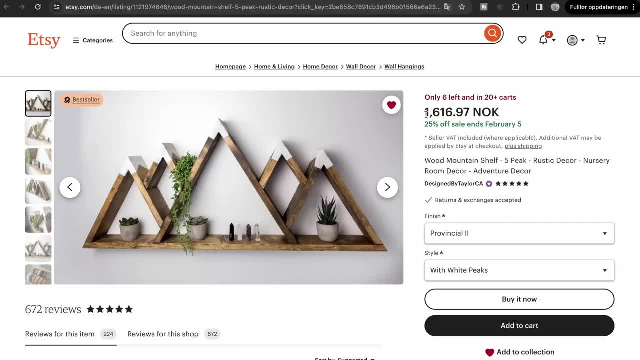 really cool shelf and it's selling for 160, $170.. It looks like, I would guess, one by four inch boards and probably maybe 30 degree cuts. The size is 36 inches long and five and a half inches tall And it said in the description that it has pre-installed sawtooth hangers for easy. 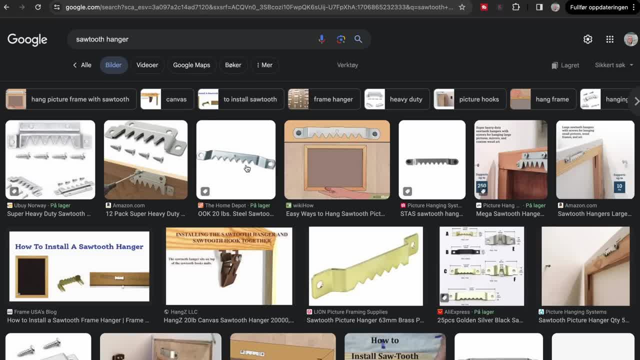 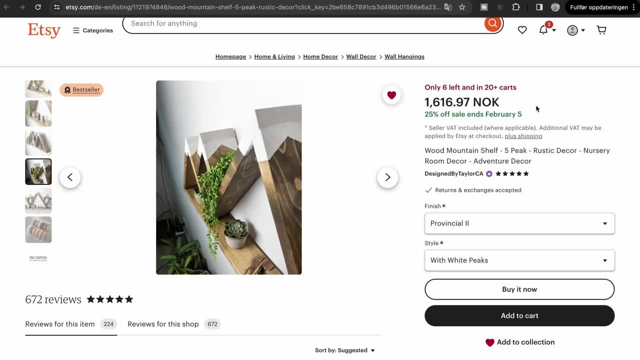 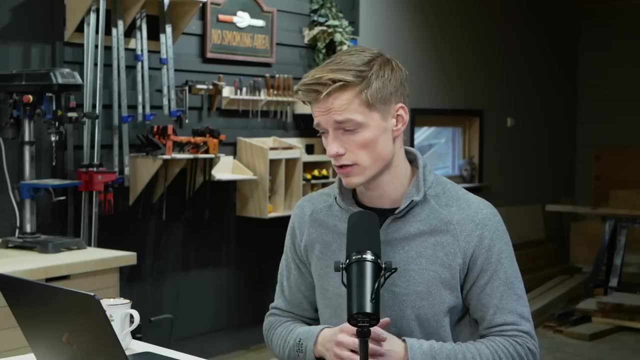 hanging. So that is these things here, Very easy to install on the shelf and also to hang up on the wall. $160, $170 per piece And that is at 25% off, which means that they're originally selling for $220 around that- Probably a little bit longer to make than the other products that 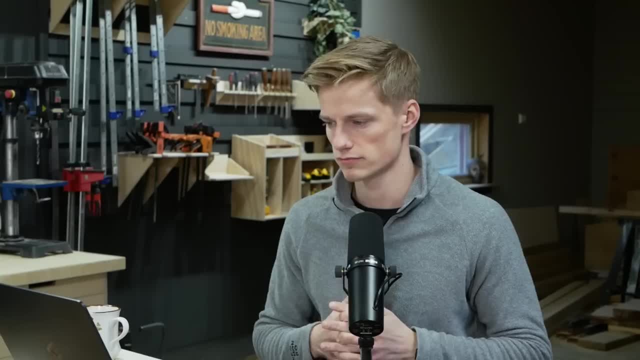 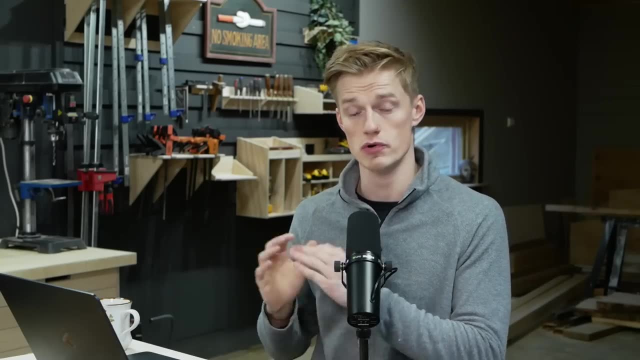 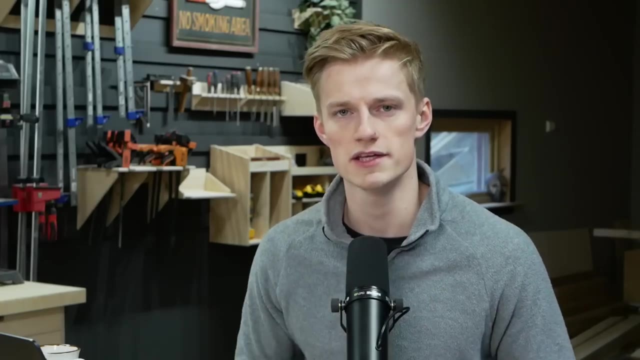 we've looked at, but it's wood and glue and nails probably. Number five is a project that I have been selling myself And, in fact, my grandpa used to make these as well. He was a woodworker, or he is still a woodworker. He's still alive and he could easily make a full-time income selling these.